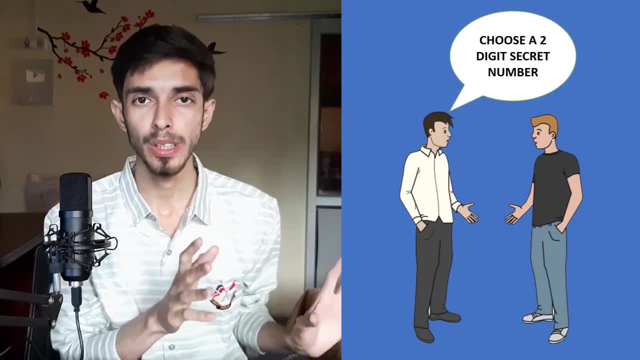 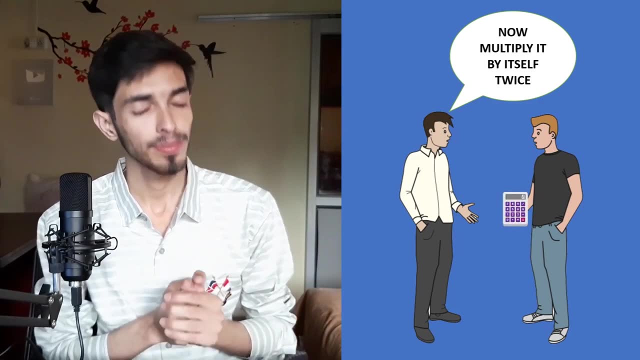 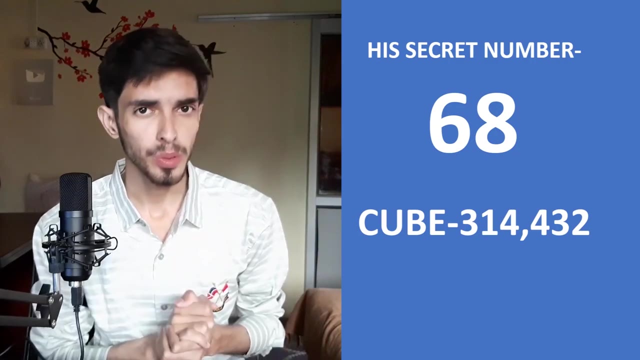 choose any two digit secret number that he won't tell you And then, by using a calculator, cube that number Like: multiply it by itself two times. Okay, so let us say he chose the number 68 and it's cube is basically 314432.. Now tell him to tell you this answer, which is 314432.. 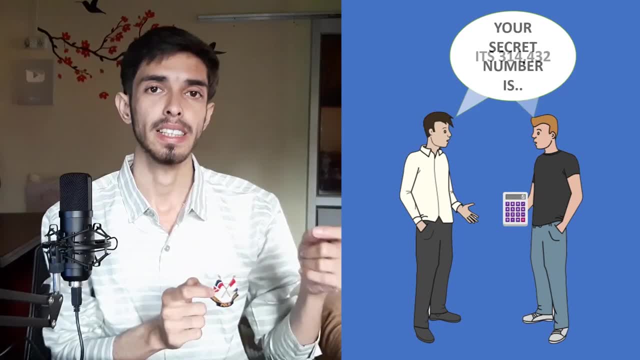 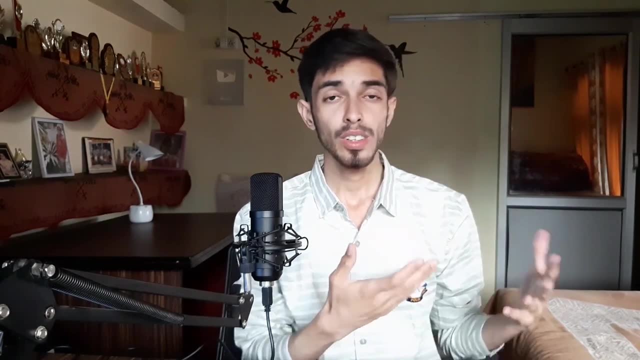 Okay, now, with this answer, you will tell him his secret number. So the only thing that you need to do is to find the cube root of this number. So let's learn it Now. the first thing that you need to do, similar to which we: 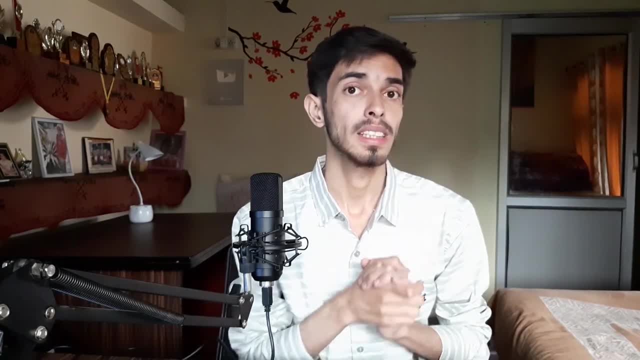 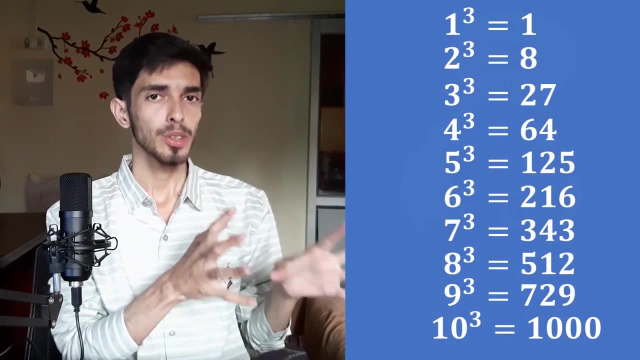 have also done in our square root video is to memorize the cubes from 1 to 10.. So here is the list of the cubes from 1 to 10. It won't take you much to memorize them Now. another thing that 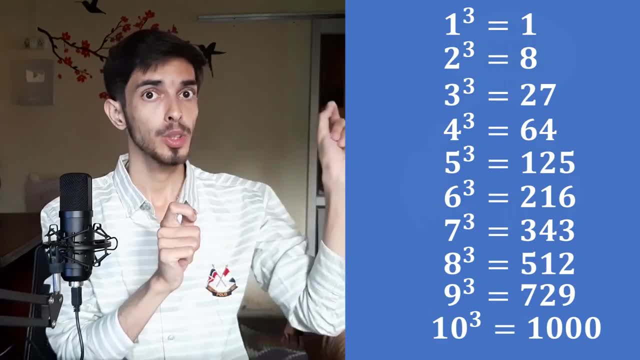 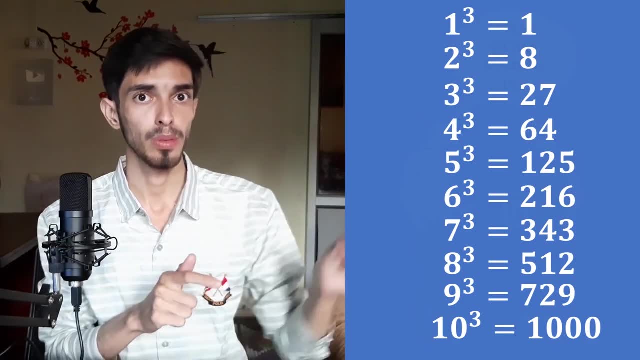 you need to focus in this is that with what number the cube is ending. and it's really easy, because for some numbers the cube is also ending with that same numbers, For example, for 1,, 4,, 5,, 6,. 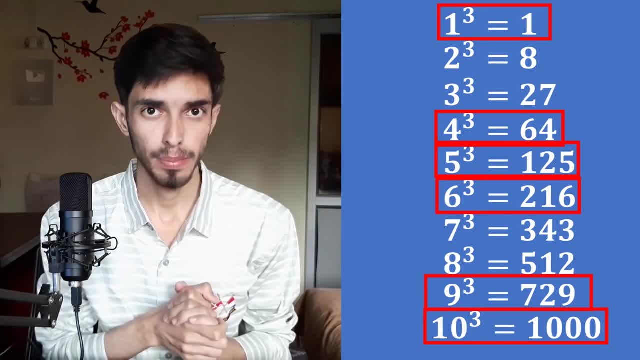 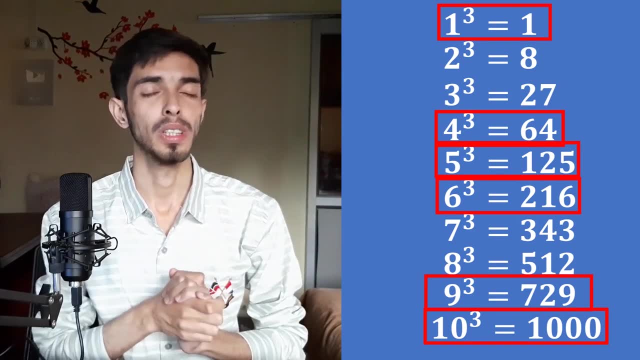 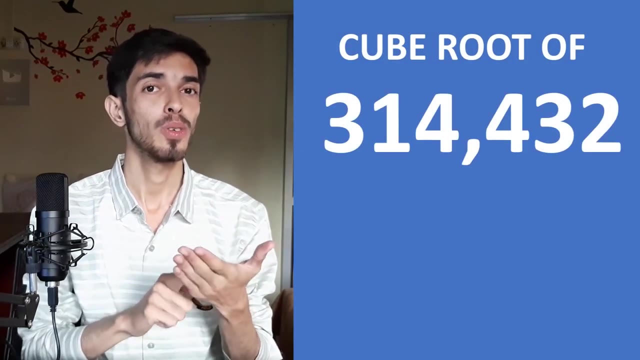 9 and 10, the cube is also ending with that same number. So take a minute and memorize this list, and if you can fluently memorize this list, you will be able to do the trick really, really fast. Okay so, if you have memorized it, now let's find the cube root of 314432.. Okay so, it is really. 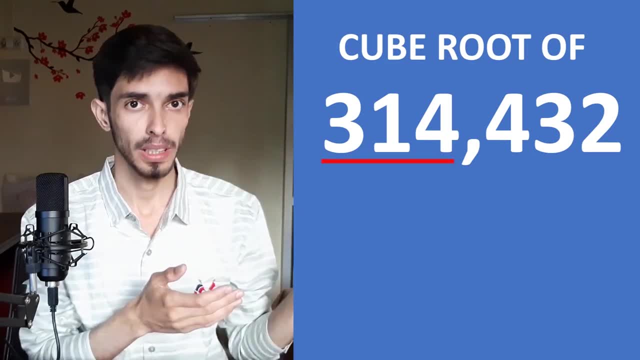 simple. Now the step one is to look at the cube root of 314432.. So let's find the cube root of 314432.. So let's find the cube root of 314432.. So let's find the cube root of 314432.. So it is. 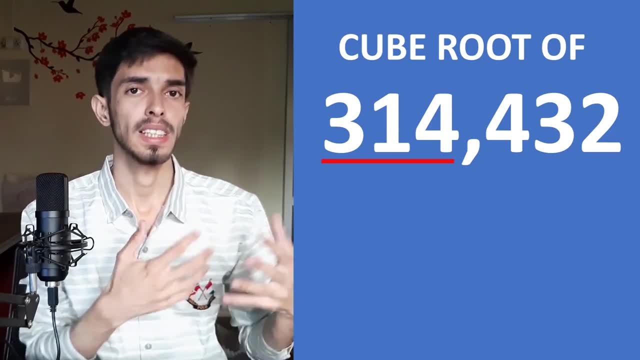 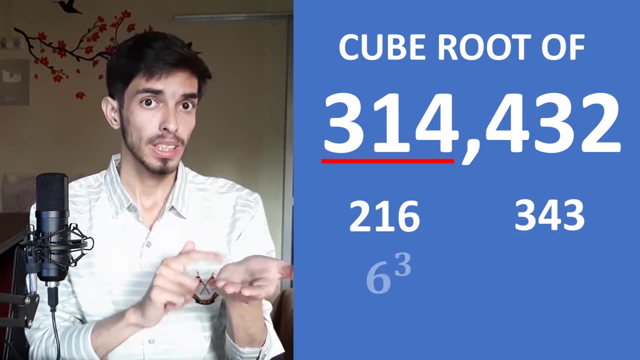 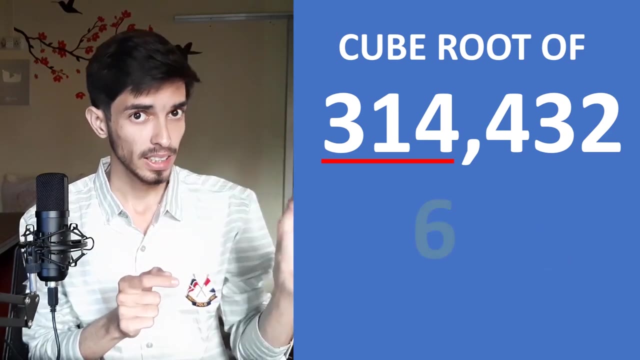 314000.. So look at 314, that is 314.. Now it lies between 216 and 343, which are for 6 cube and 7 cube. So the first digit of our answer is in 60s. So the first digit is 6.. See so easily we have. 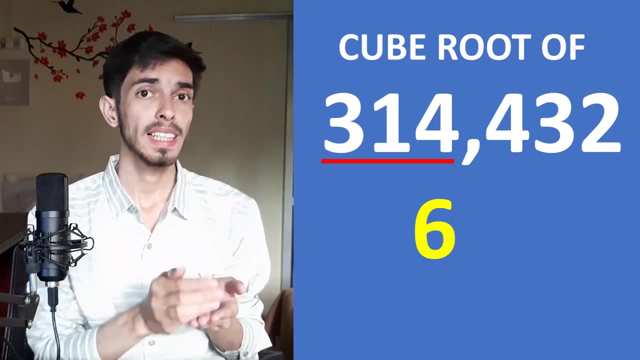 got the first part of our answer. Now to determine the second digit, see with what digit this number is ending, which is 2.. Now let's find the cube root of 314432.. So let's find the cube root of 314432.. So 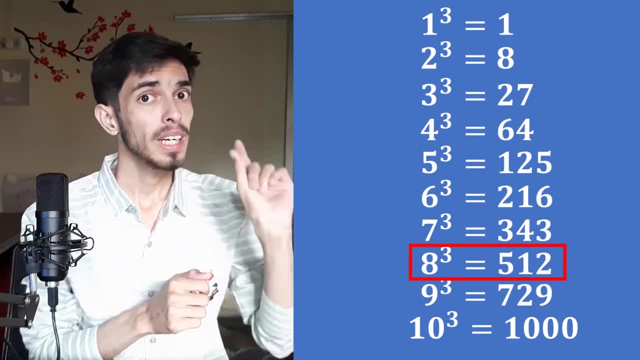 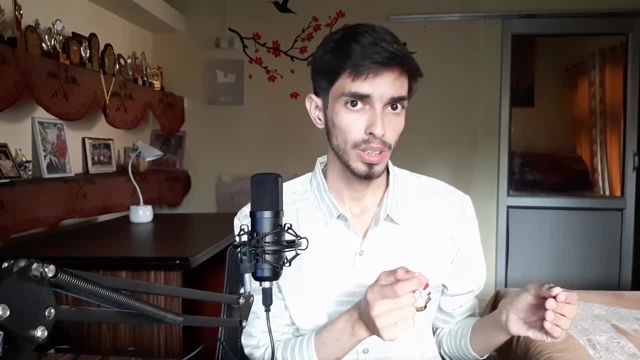 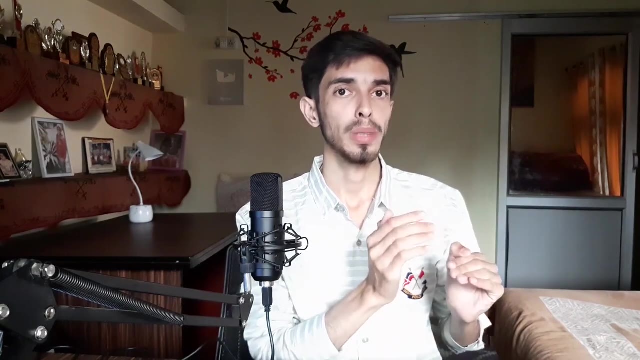 see which cube ends in 2.. Only 8 cube ends in 2.. So the answer is 68.. Now, one thing that I want to tell you: that while learning square roots, there were numbers that were ending with same digits for different squares. So we needed to devise a new method to determine which one to